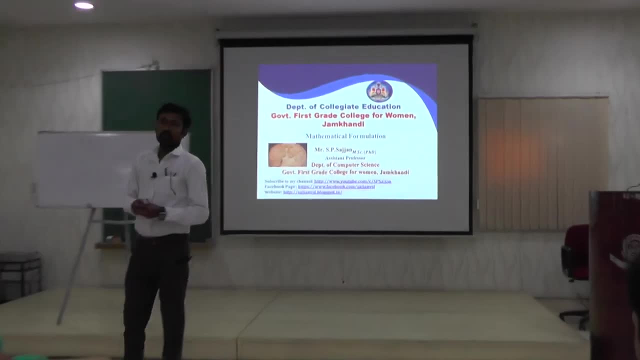 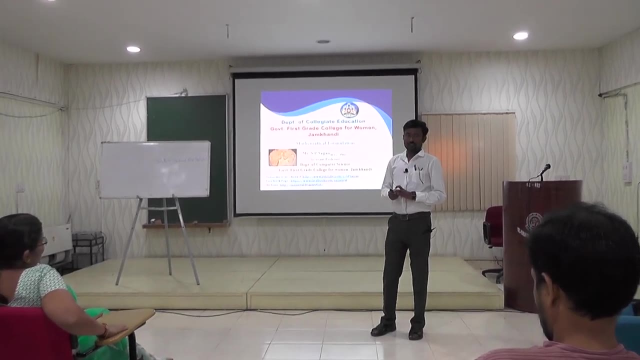 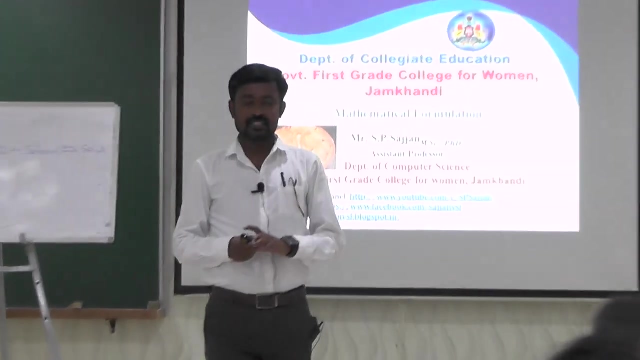 Good afternoon. one second, My initials: SP, Sajjan, Government, First Grade College, Jamkhandi. I have selected somewhat different topic. It should be useful for all. It may be commerce, it may be science, it may be management, except I think somewhat actually language also it is useful. 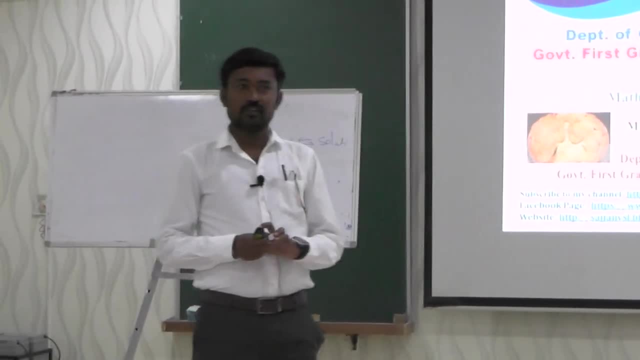 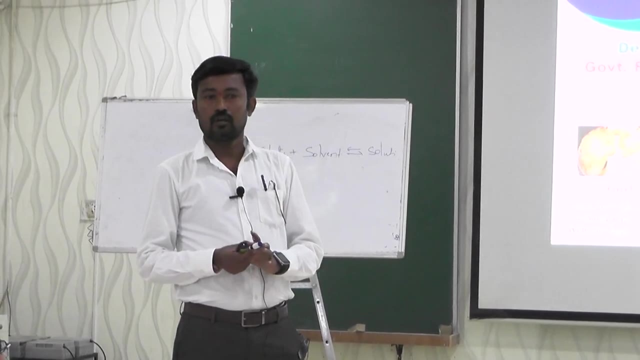 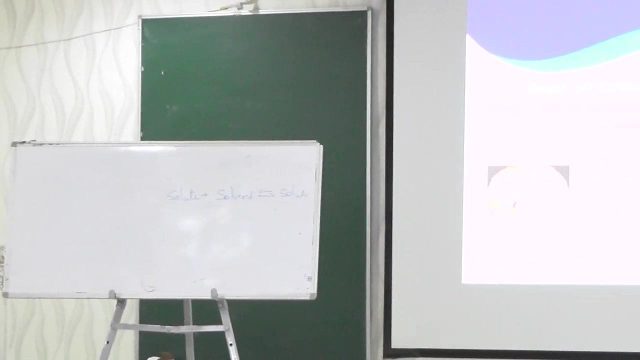 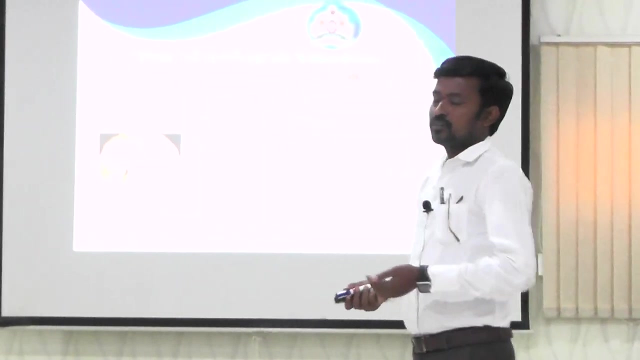 Fine art also. actually, fine art is useful for mathematics, Mathematical formulation. Anyhow, already we are all our assistant professors. Now we need to move somewhat for research. In research, first step of the research is identify the problem. Anyhow, we are very well known, we are daily life. we have come across so many problems. 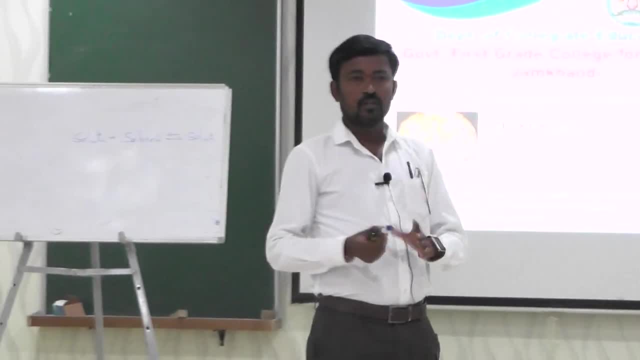 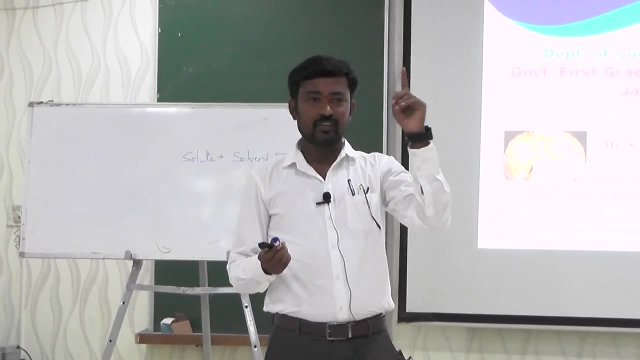 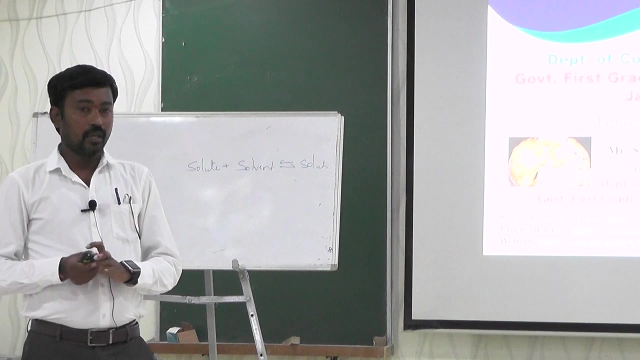 Everyone is facing so many problems I hope all of you are aware of at least you are facing one problem. No one, I think Anyone. You don't have any problem. Everyone has many problems. But now our aim is to convert that problem in the form of mathematics. 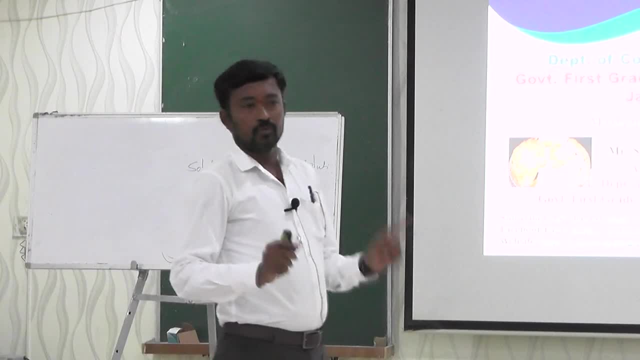 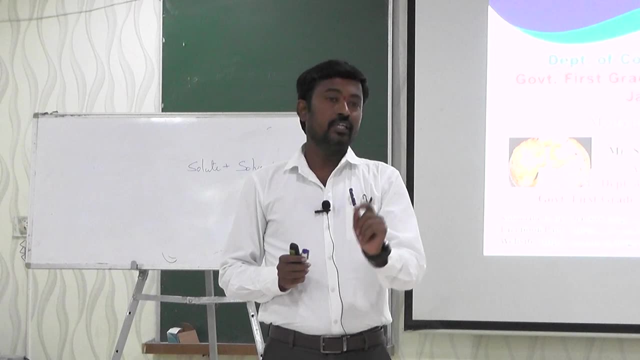 There is one statement: every real world problem, you take it. every. that is very important. Every real world problem convert in the form of mathematics, then only it is a solvable problem, Or else it is unsolvable problem. You may take it. 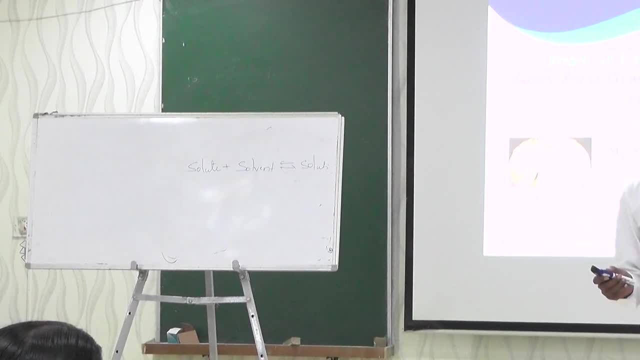 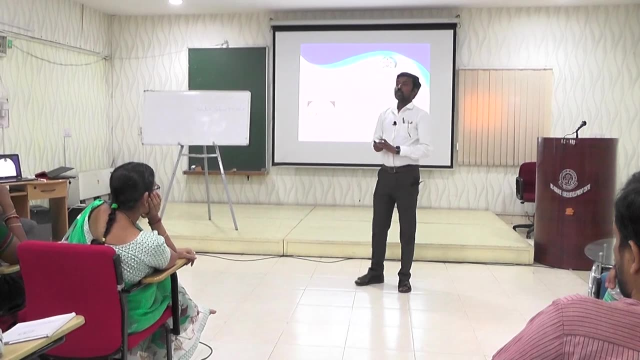 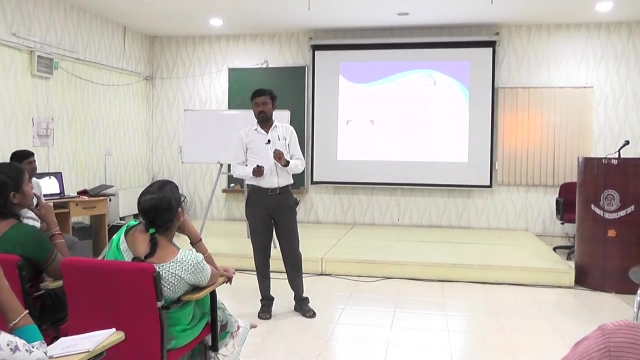 Preparing upma, or you take it any real world problem, it should convert in the form of mathematics. Then only it is a solvable problem or else unsolvable problem. Today, my this class objective is to. I have taken very simple two examples, real life examples converted in the form of mathematical model. 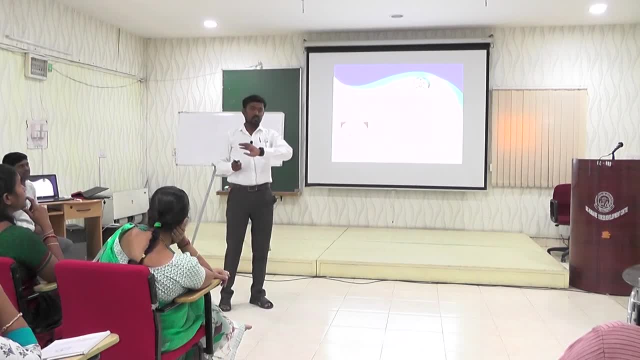 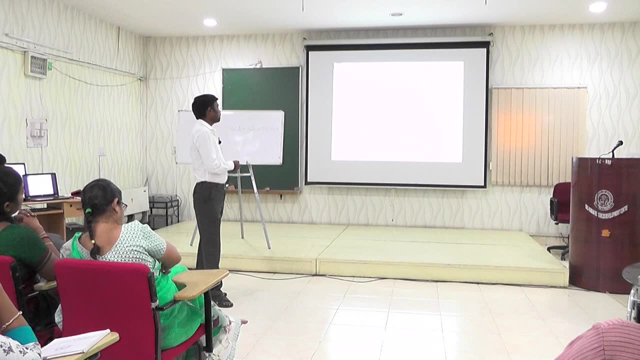 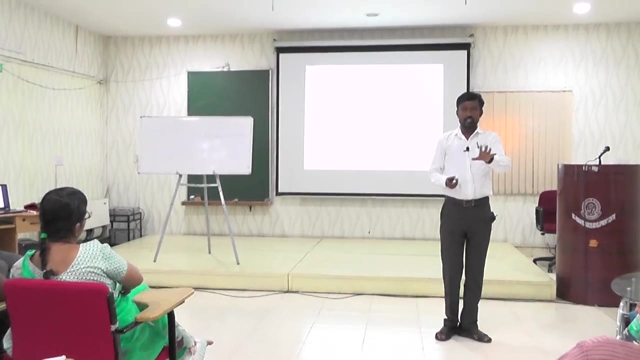 I hope all this model is familiar with all management, commerce, everyone. So first, first of all, before defining problems and all, just what is mathematics Can you? can you define anyone? Because we have studied fifteen year or ten year, at least ten year, mathematics. 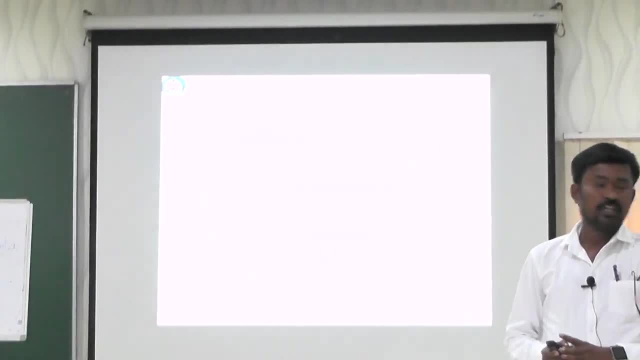 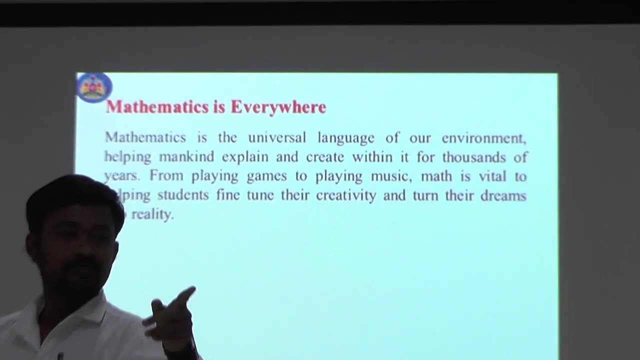 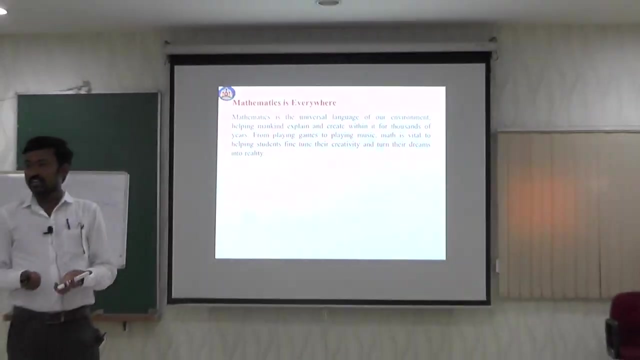 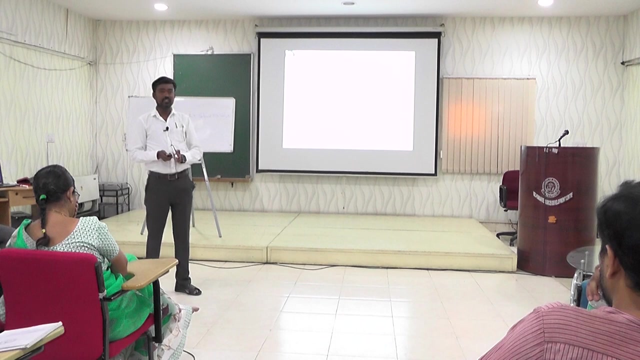 After that, some of you, science means fifteen year mathematics. Can you define anyone? what is mathematics? Mathematics is a problem: Calculate It is not possible to define in one sense Because it has so many dimensions in mathematics. For looking this first statement, it started. 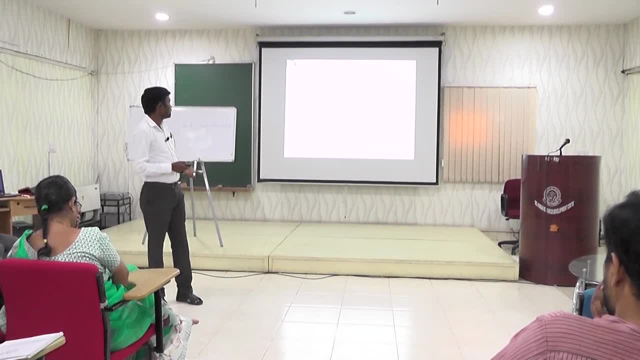 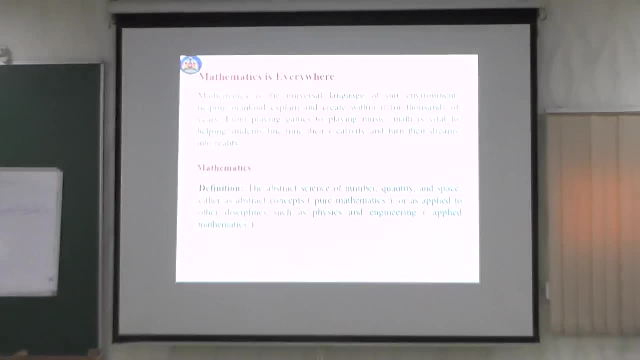 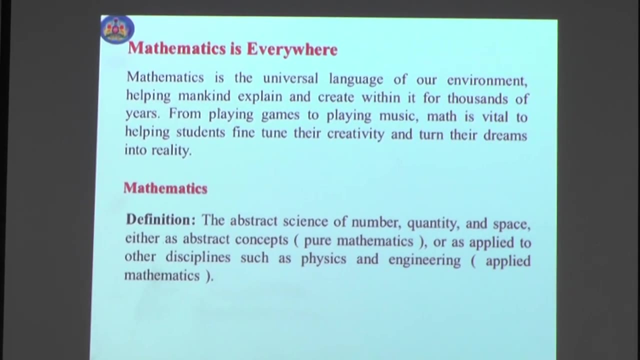 But anyhow you may take it, one definition of mathematics is the abstract science of number, quantity, space, either as abstract concept or as applied or other discipline like applied science, Pure science or applied science. You may take it as informally. There is no definition, means no one, as like physics, mathematics definition. 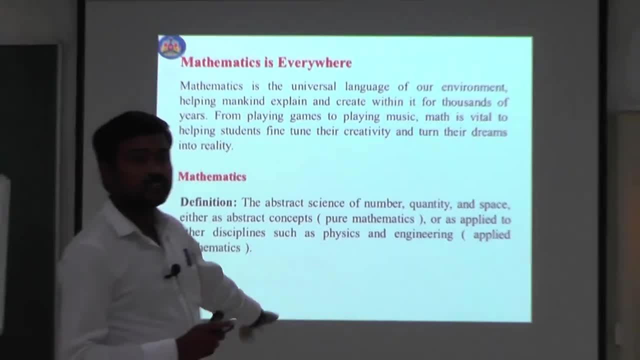 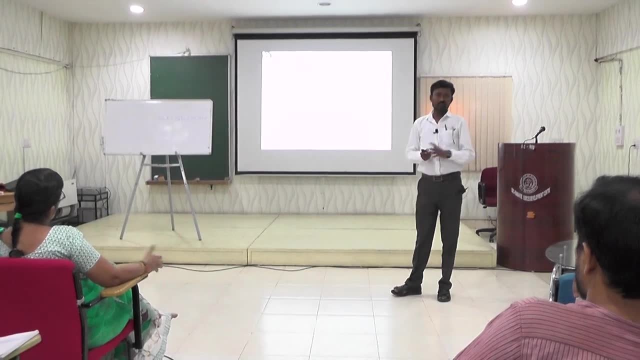 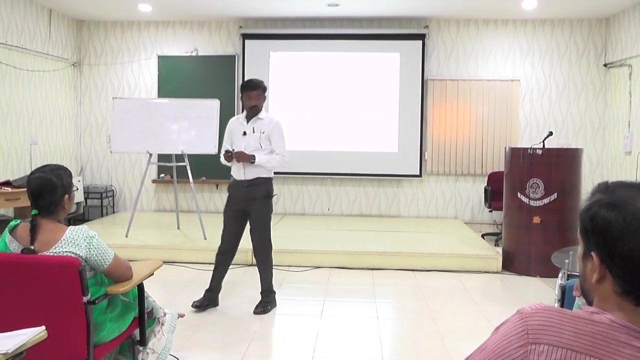 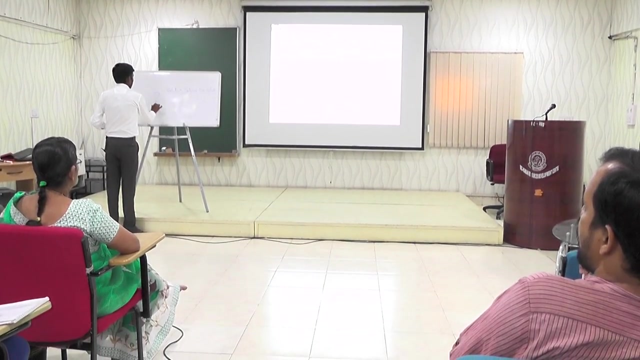 Definition. still it is. there is no fixed definition, But it is widely accepted definition. what is mathematics? Here there is one concept, one word is abstract. What do you mean by abstract? Beyond Abstract means in simple way: Who is he? 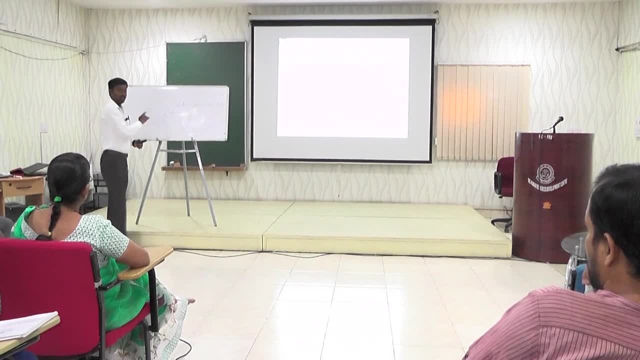 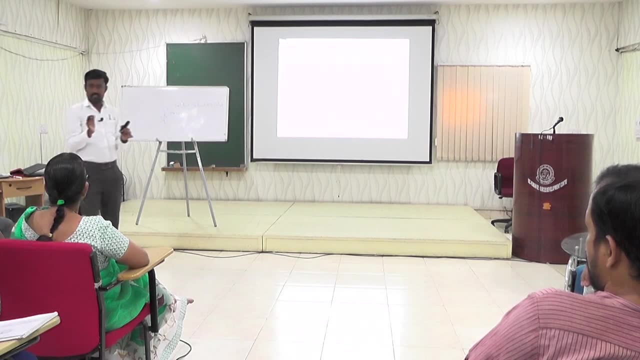 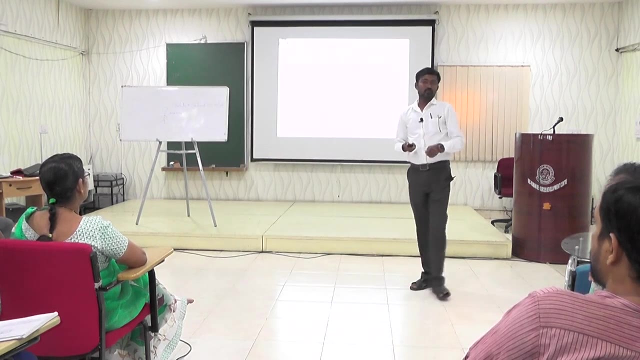 Right now. now you can touch in, But if you write simply, that is abstract. There is one form. It is physically not exist. but even though we are believing it is exist Most of the time we are in computer science and all we are explaining binaries is storing like this: 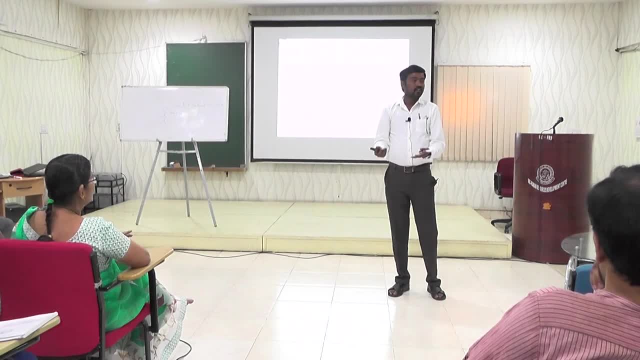 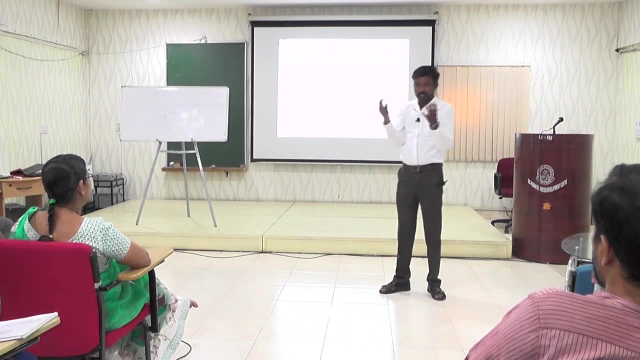 It is in a memory. It is storage zeros and ones, everything. But if you told, ask me how it is exactly storing. it is not possible to show it. It is not possible to show it Where, conceptually, we are accepted. this is storing like that. 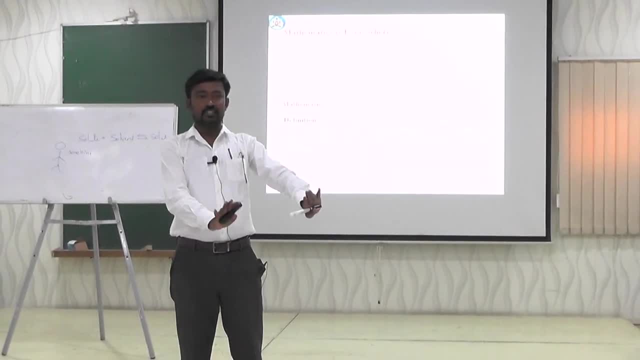 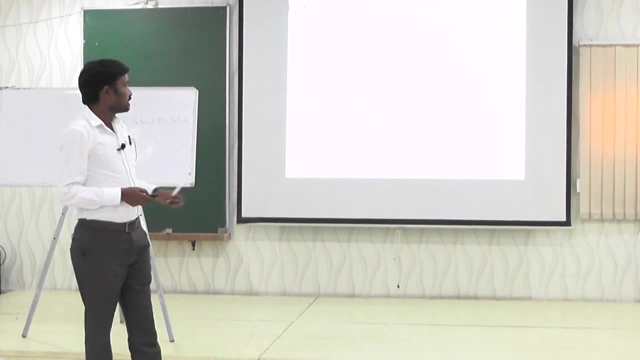 It is proven, It is working like that. Widely we are accepted It is. maybe it is storing like that. We don't know, No one knows. No one seen exactly what it is. This is exactly what is mathematics- Mathematics. anyhow, it is universal language. 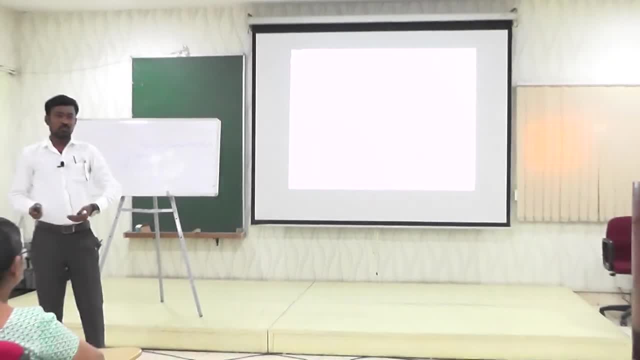 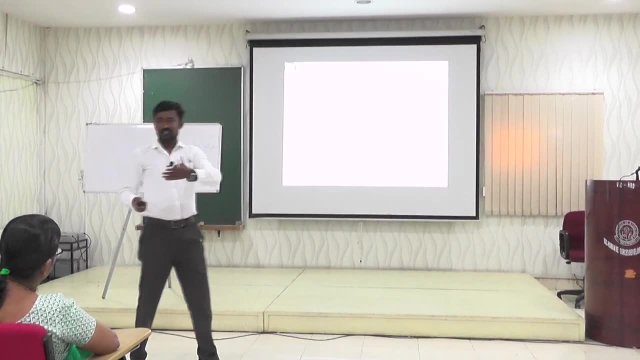 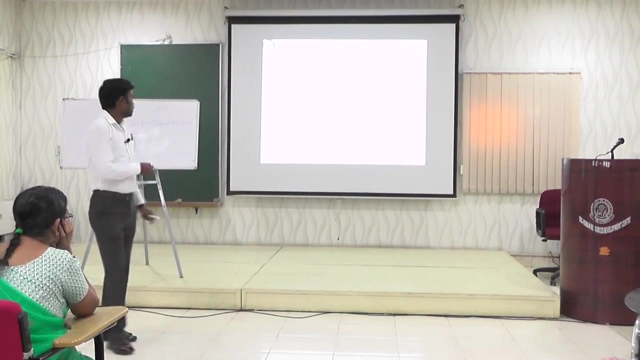 Every subject without I think today is almost all subject. you take it economical, You are used surplus, less than greater than something In commerce, and madam has taken gates, logical gates, and all comes under mathematics. Now my object is to- I will take one small example- abstract, that is, definition of abstract. 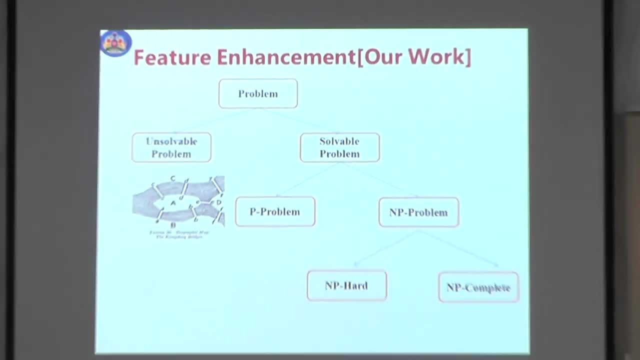 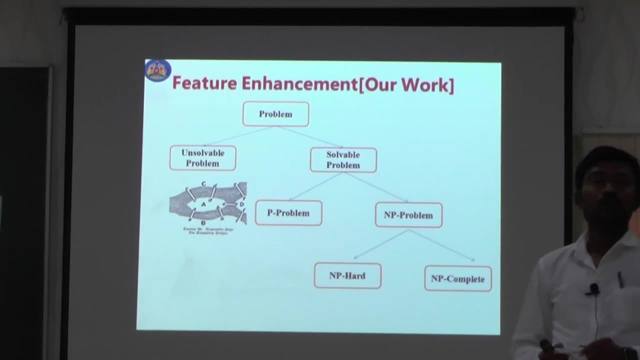 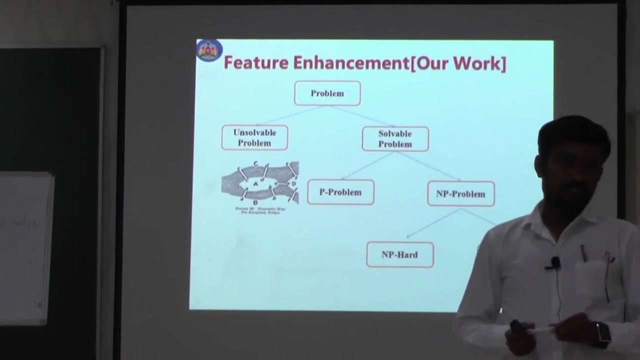 This is exactly total problems in real life, divided into two major parts. One is unsoluble problems and soluble problems. There are 26 unsoluble problems still exist, million dollar questions. You may go and find it. You may go and find in a clay mathematics website. 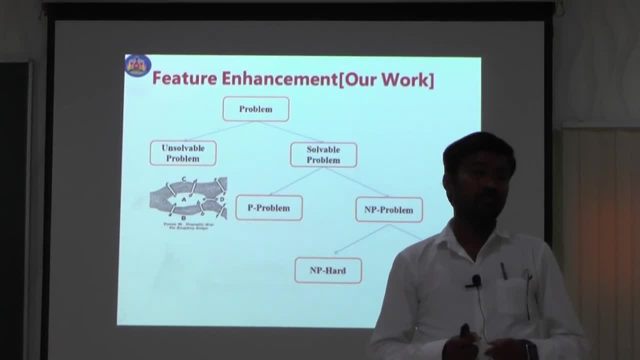 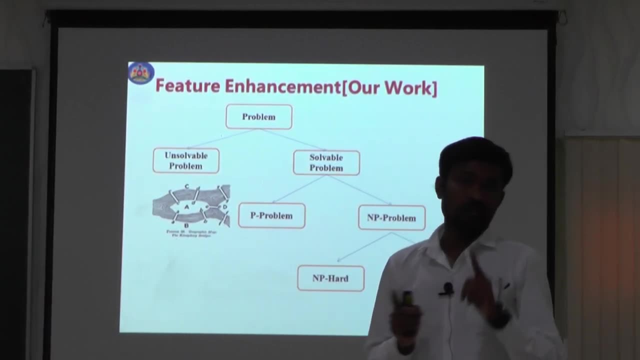 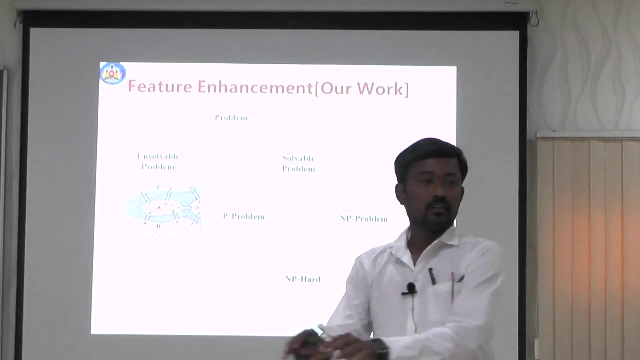 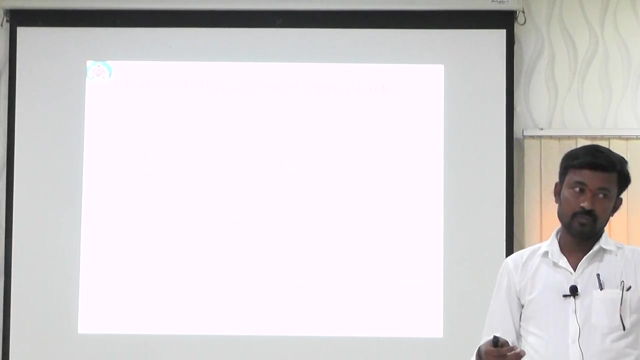 There is a website, clay mathematics. They are listed Initially. they have listed 41 unsolved problems. Already it is solved. nearly 15 problems are solved. If you solve one problem you will get a million dollar, Million dollar problems. It itself is: you may type in Google million dollar problems. you will get 26 unsolved problems listed in clay mathematics website. 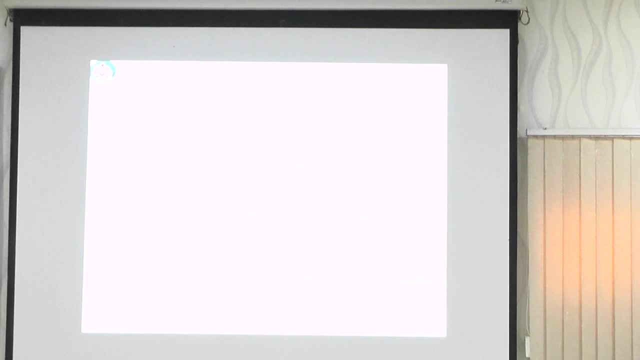 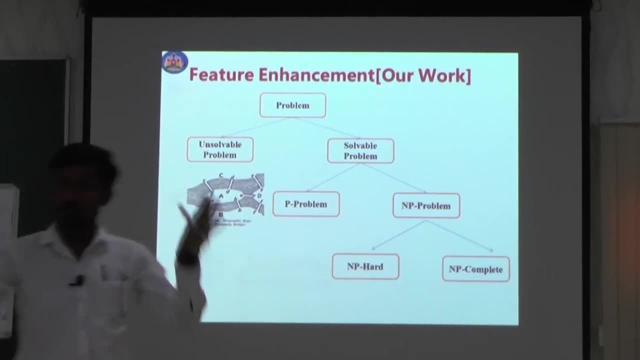 You may go through it. Okay, If you solve one problem in computer science related n is equal to npr. not Leave it, I will not go in depth. Then only problem. everyone know the. what is the problems? Problems divided into two parts. unsoluble, soluble. 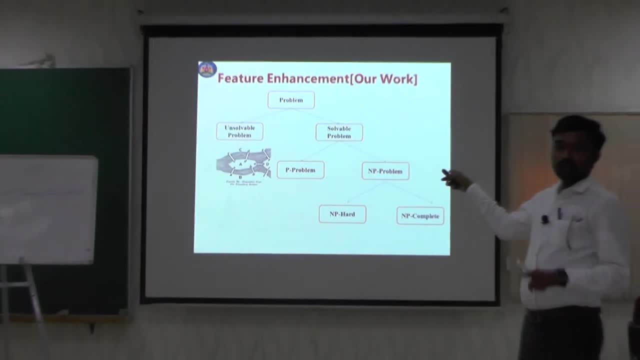 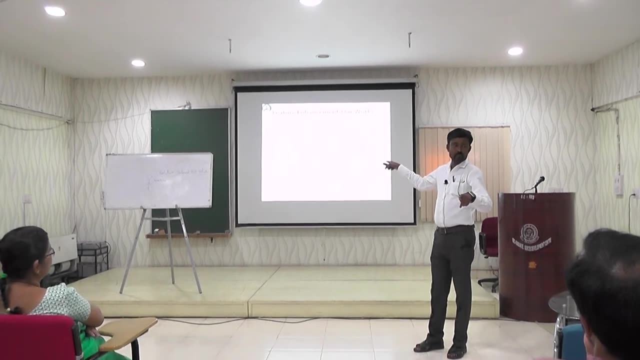 In unsoluble. best example is: I hope everyone saw that graph in 10 plus 2 level or 10 level Coins bridge problem. Coins bridge problem. It is still. it is unsolved. Okay, It is proved, it is unsolvable. 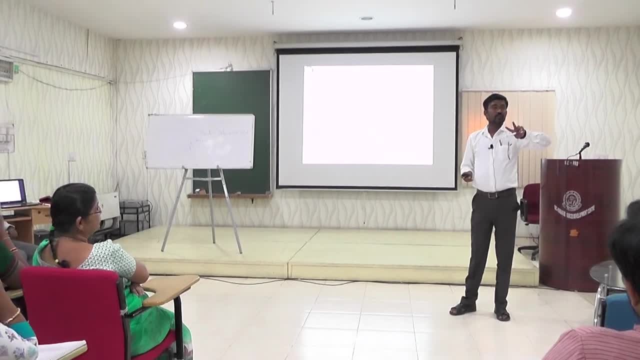 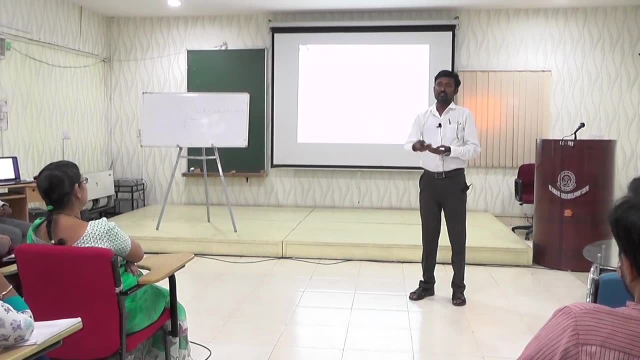 Leave it Now. come to the solvable problem. Solvable solvable- two types. Some problems you may solve in a small amount of time Means what we will get a result after one year or two year. This type of problems comes under p problems. 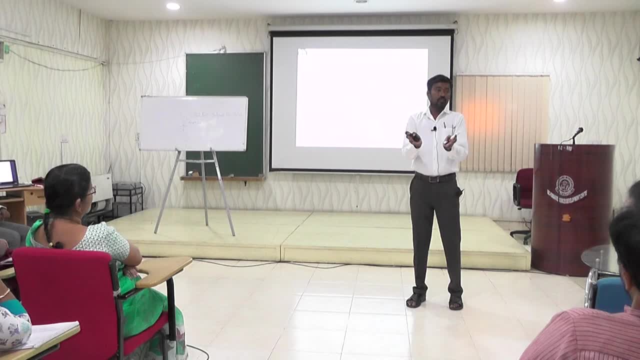 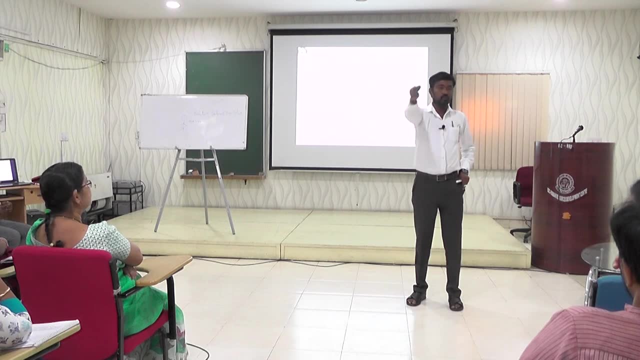 Okay, Some problems. there is a solution, but it is not possible to tell. there is, For example, one example. I will tell you: In 2090, there is a function in our home. You should, you all should, come in our home, In our home. 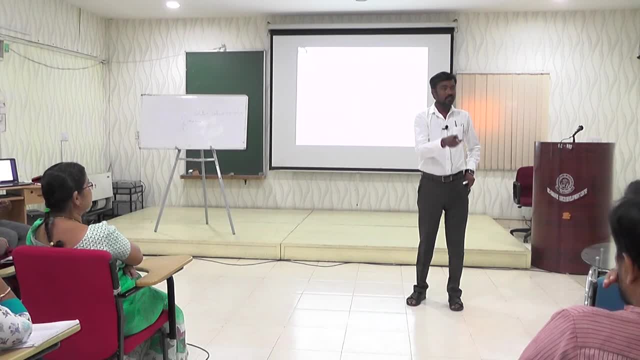 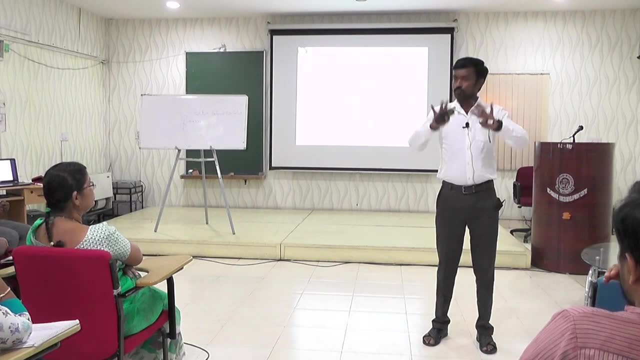 Can you tell the answer now? But it has a solution or not? Problem has a solution In 2090. there is function in our house. You should all come What you will tell First of all in 2090, if you there. 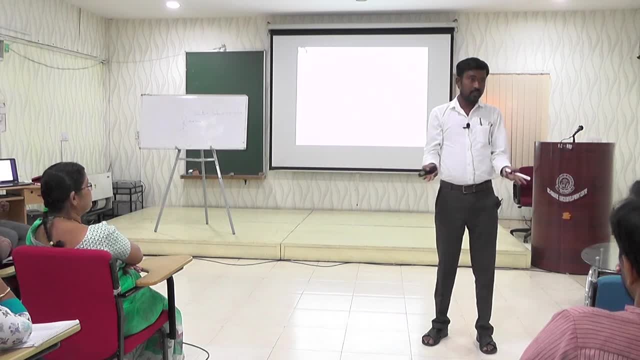 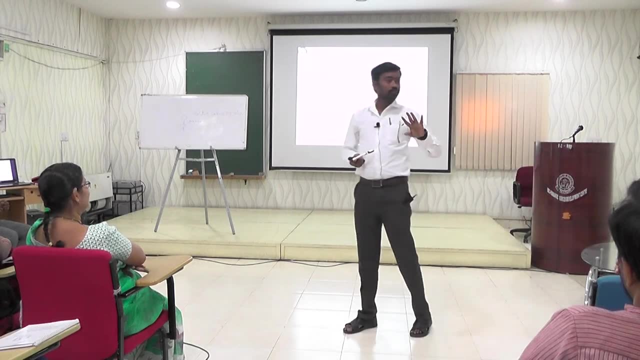 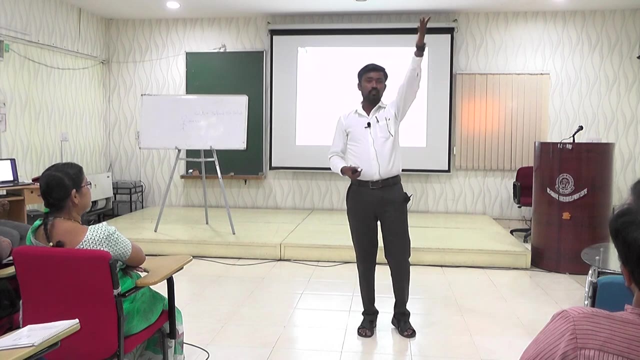 If I will be there. We will see later on, But not decide at present. That type of problems is comes under can be hard problems. It is problem has a solution. Problem has a solution, but not possible to decide at present. You may, problem will get a solution in 2090.. 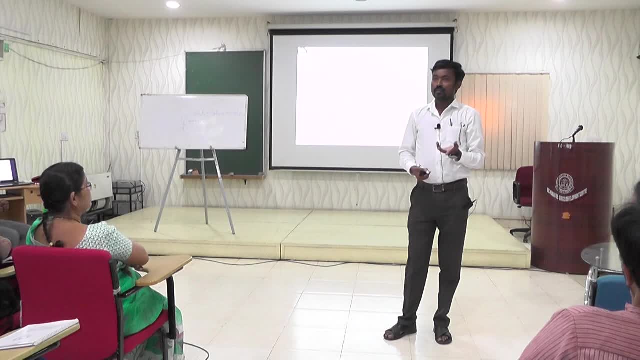 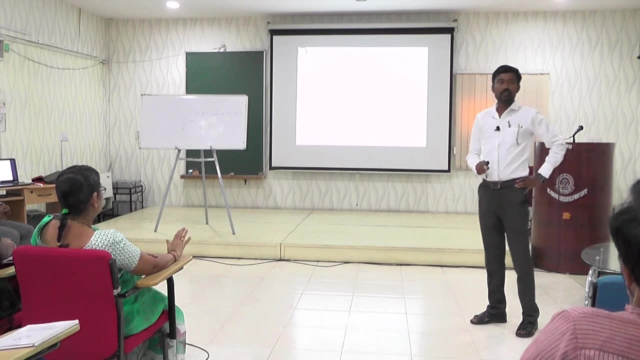 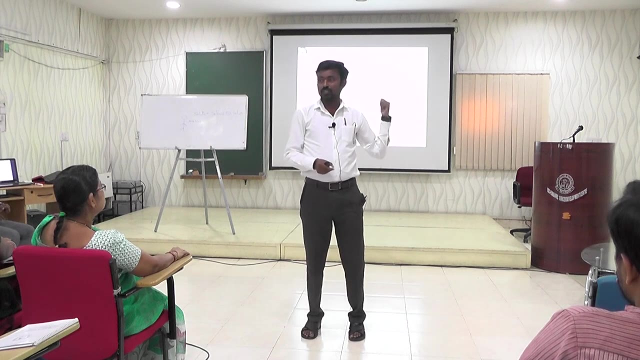 You will attend or not, You will get a solution, But at present there is no answer. That type of problems are NP hard problems. Some problems are NP complete problems. These are the problems are. takes so much time, it will complete, But I will show that example. 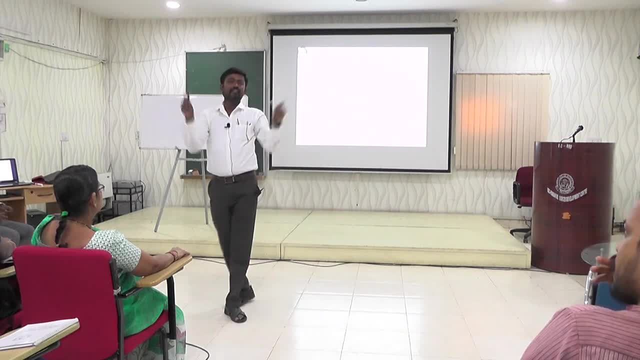 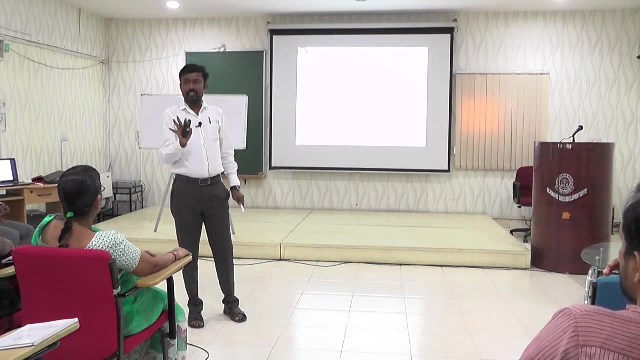 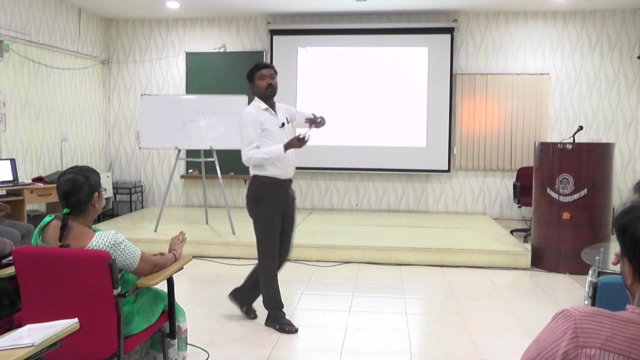 Okay, Is it okay? So just for like, How many problems, How many problems? And in day to day life, It is not only for mathematics, It is for every subject. Total problem is divided into two part. Again, It is soluble, means minimum amount of time. 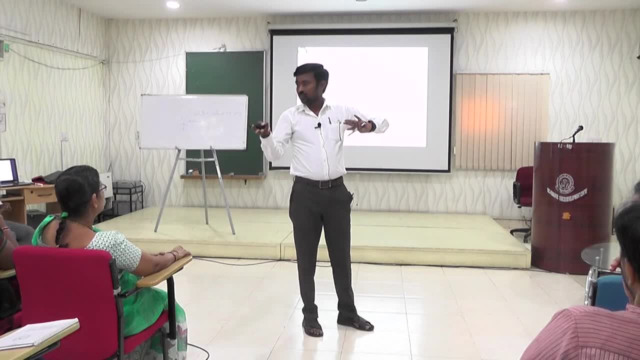 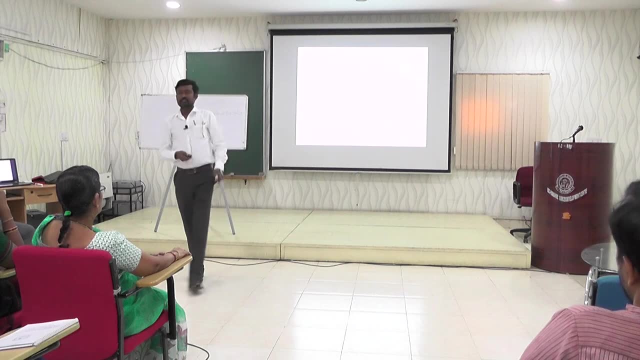 Some problems are, it takes more time, Some problems are difficult to predict at present. Okay, Then we will go, for I have started journey. Jamkandi And I came to Vijayapura And Putigi- It is in Maharashtra. 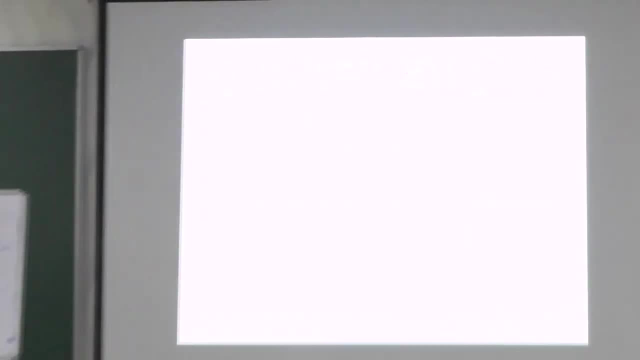 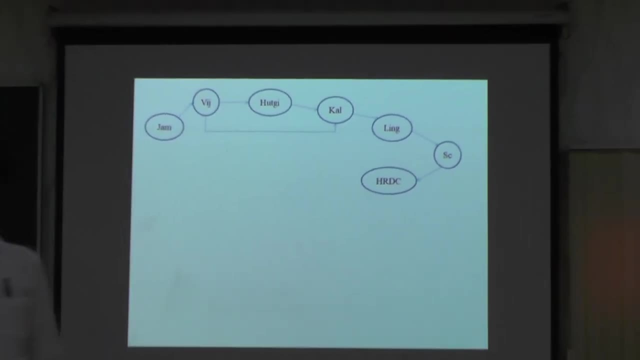 And I came to Kalburgi And I came to Lingampalli And Secunderabad, Then SRDC- Okay, Actually Gacchipalli. I missed Because it is, It is, It is not- came in the train path. 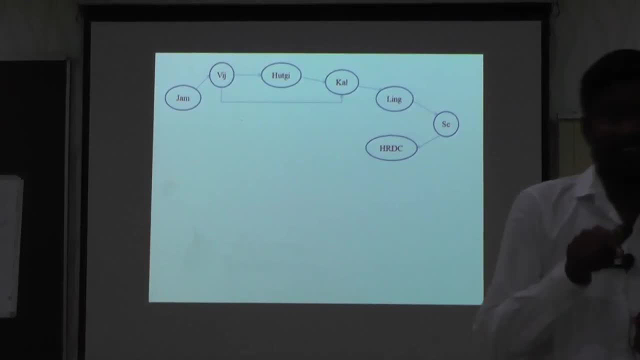 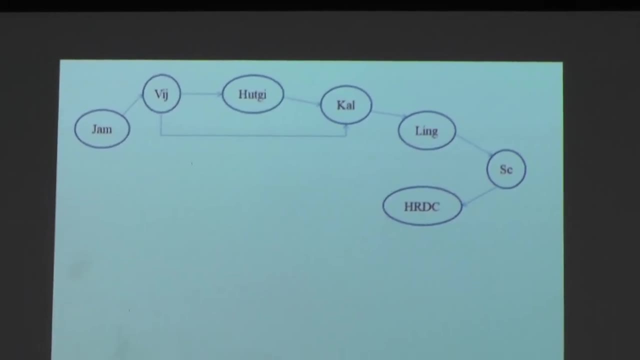 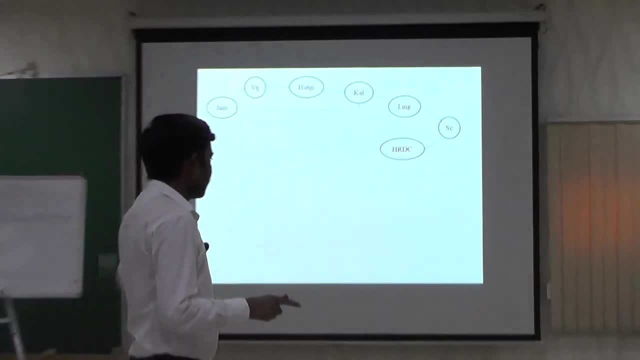 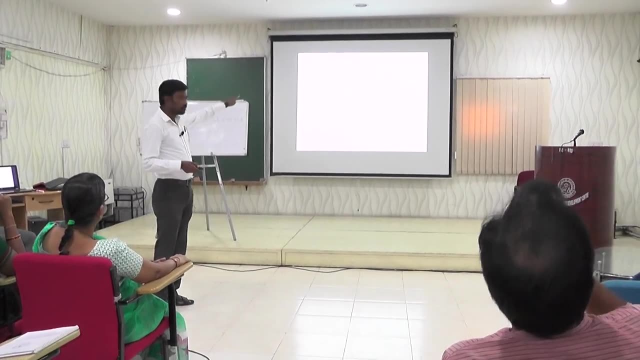 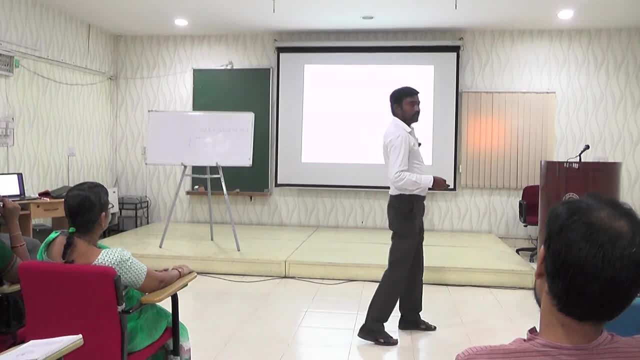 Vijayapur to Kalburgi. You see it, One more path is there. I may come to the Jamkandi, to Vijayapur, Vijayapur to Kalburgi, And I think Which path- this one, Whatever- I have selected? 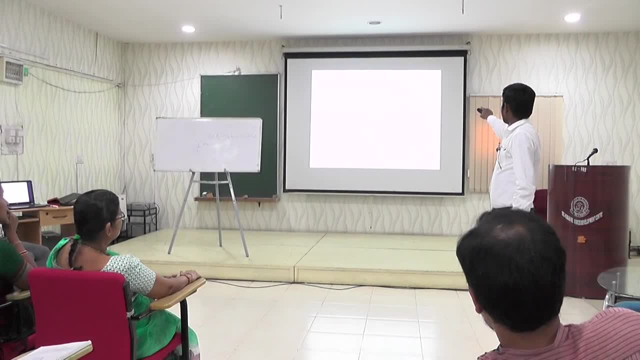 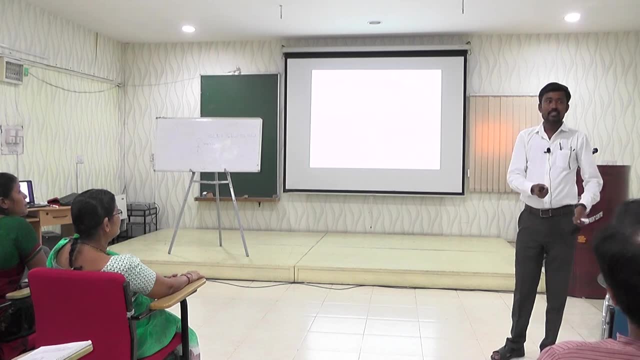 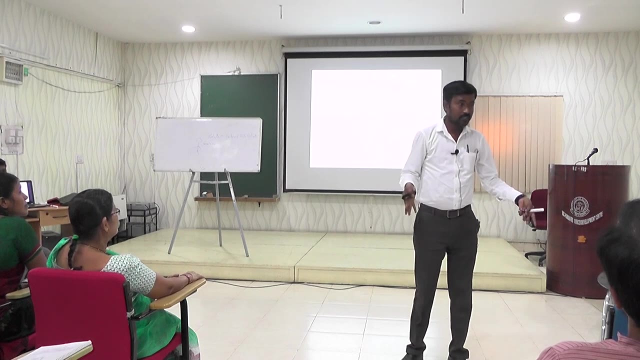 That is train path, Okay, But I may came Jamkandi to Vijayapur And Kalburgi And Lingampalli Or may be SRDC. Okay, In that, How you will select Paths In Google map. also give two to three paths. 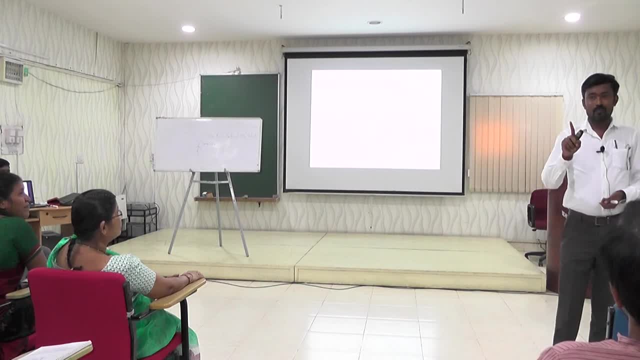 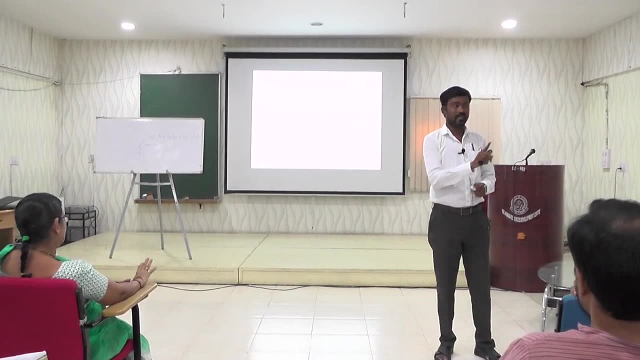 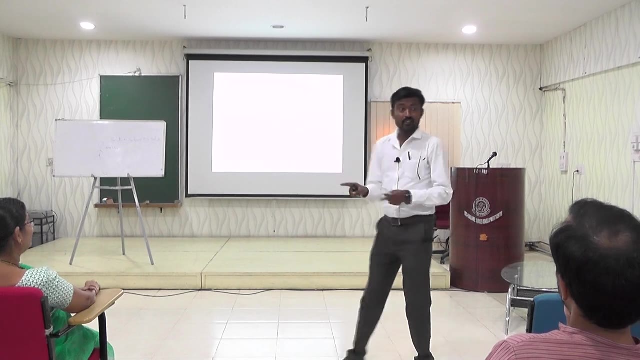 In that How you will select the best path. One is Distance: Distance, First, Timing Timing Distance: Okay, Budget, Actually, I have selected. Long path Budget: Okay, Budget, Actually, I have selected. 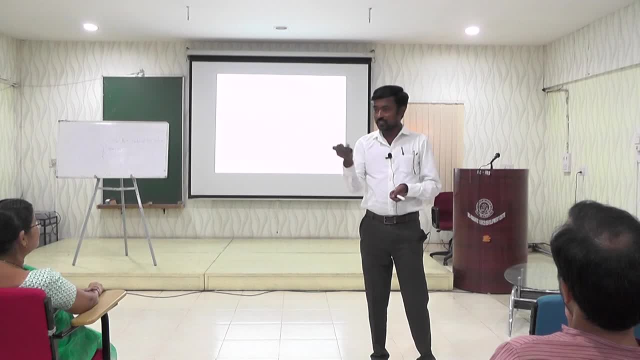 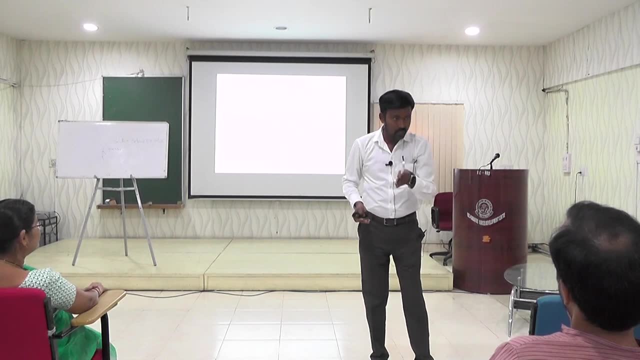 Long path, Because It is Less expensive, Because I have selected Train, I have moved to What is Maharashtra And came back to Andhra Pradesh Instead of If I came In Bus In. 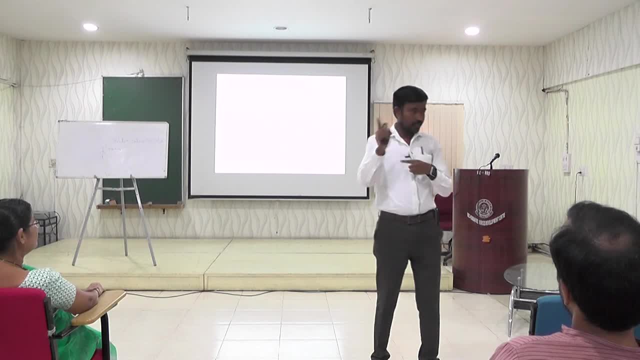 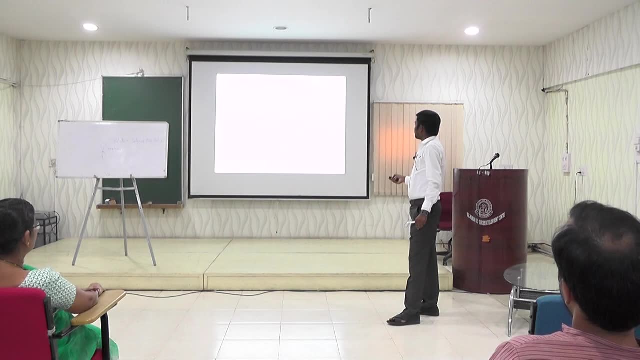 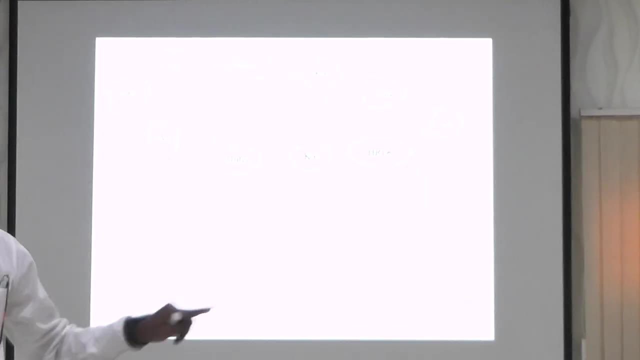 Karnataka. I can reach Here. If you came From Flight Directly, You can Reach In Wireless Also, There is a path I will reach Back. Okay, Seeing This Type Of 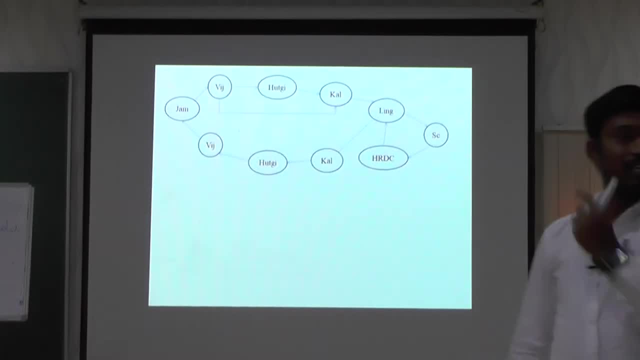 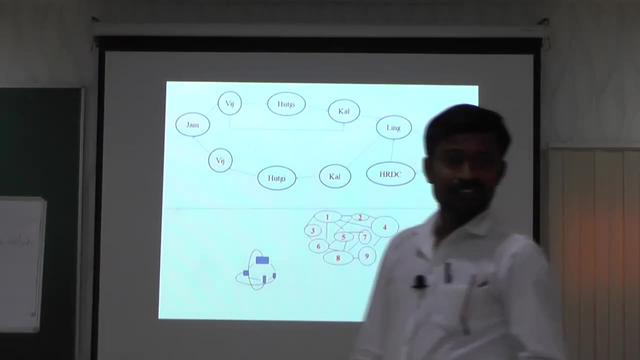 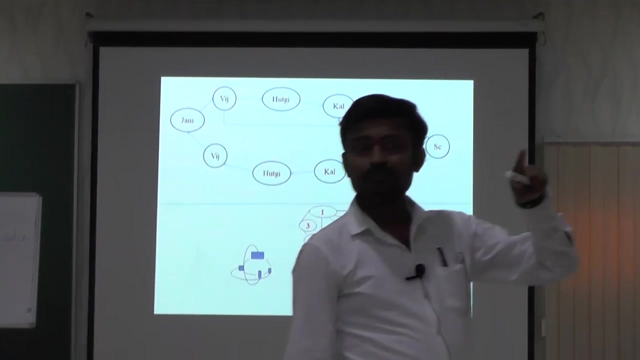 Diagram In: Up To 10. Plus 2.. At Least, Everyone Studied Mathematics. 10. Plus 2. At Least Have You Seen This Type One. 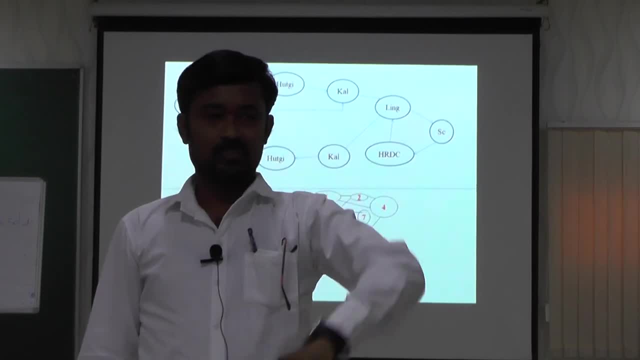 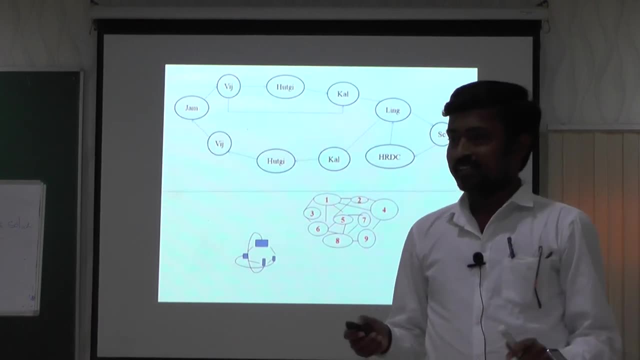 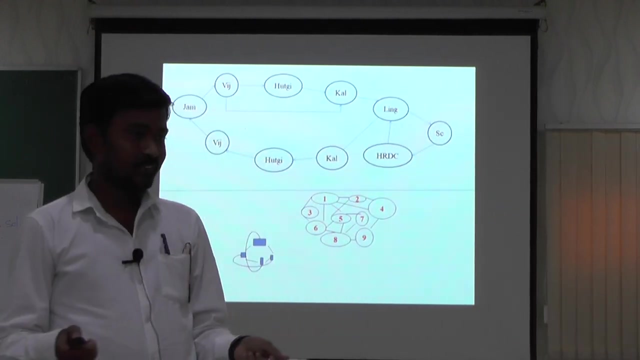 Chapter We Have Studied In 10. At Least, 10. Plus 21. At Least. Signs: Graph Theory. Graph Graph Theory. Jalakrut, Canada, Jalakrut. 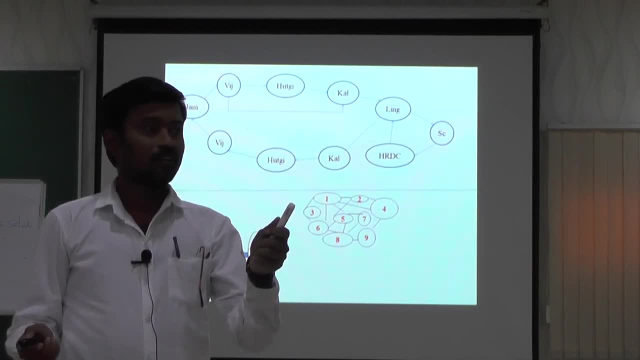 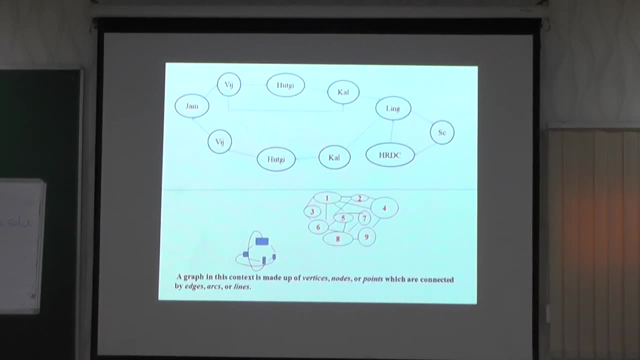 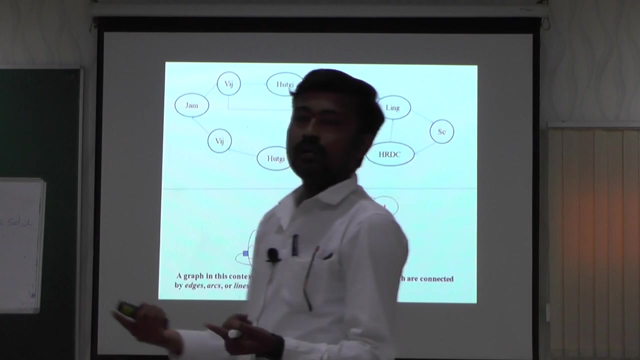 In Canada. Graph Theory, Graph, Graph Theory. It Is A Graph Theory Actually. What Is Graph? It Is Widely Used Technique To Convert Real Problems. 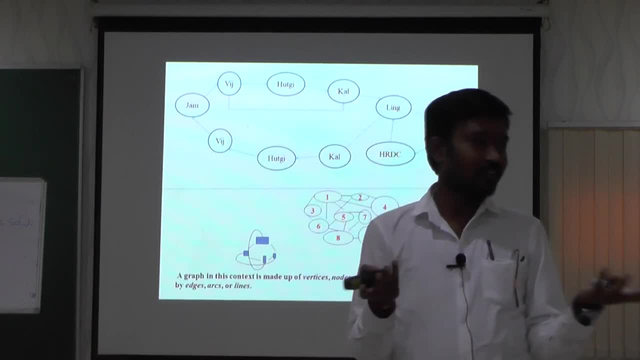 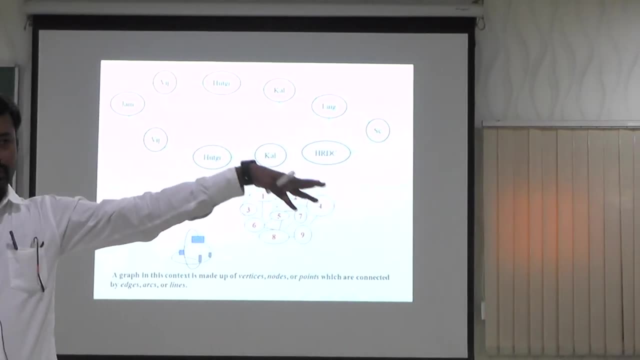 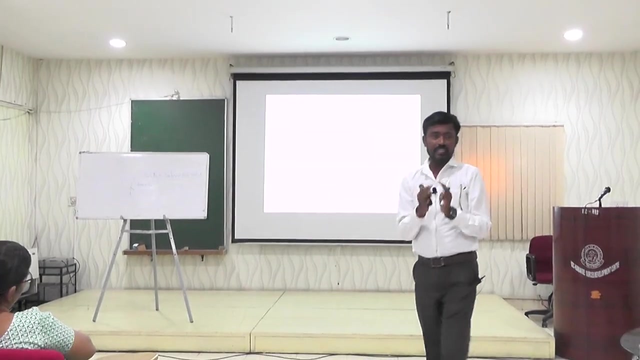 To Mathematical Problem. It May Take It As A: What Is Graph Theory? Is A Graph Theory? Is A Graph Theory Is Widely Accept Means. 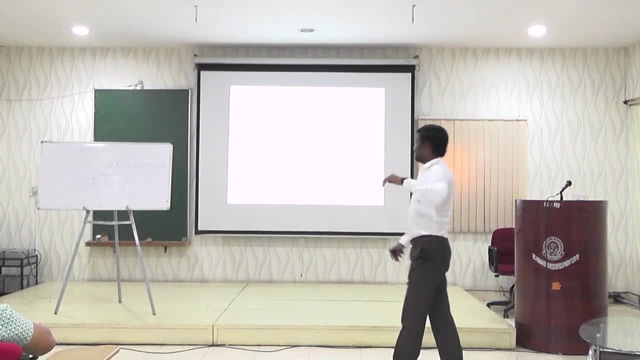 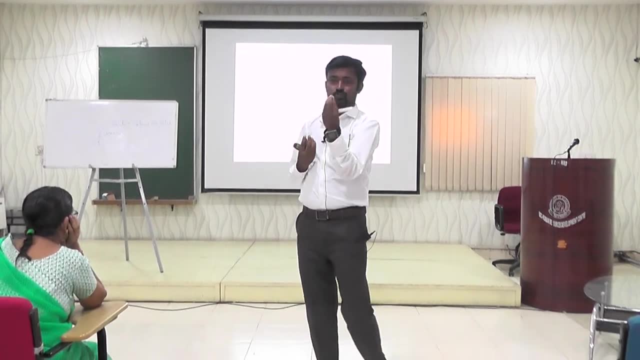 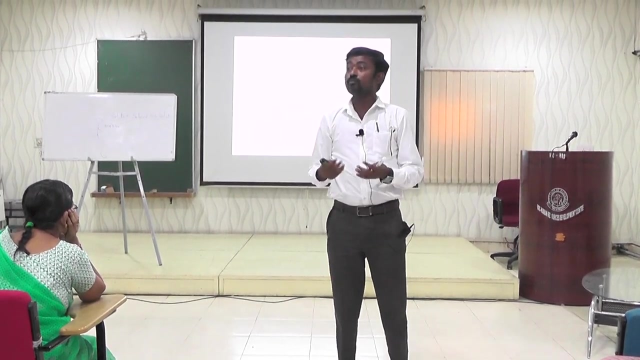 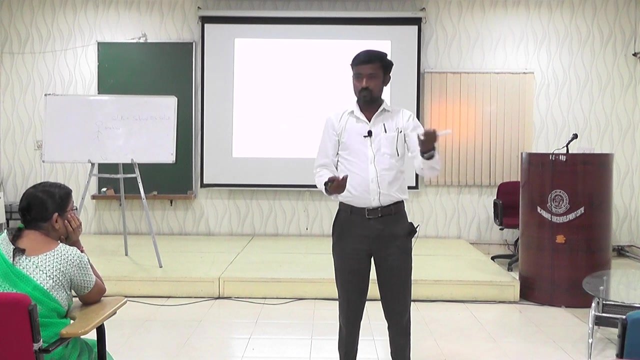 Used Technique To Convert Real Problem Into Mathematical Problem. In This To Let Us, Let Us Take One Of The Algorithms Developed In India. If I 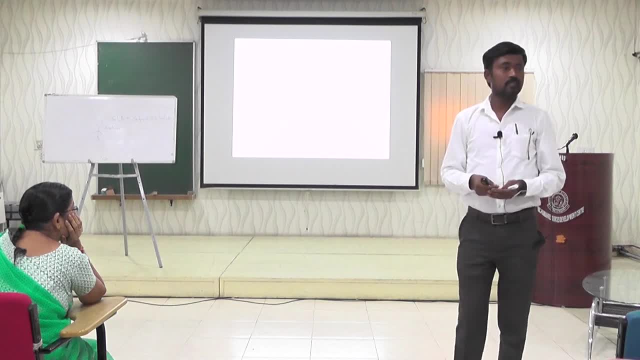 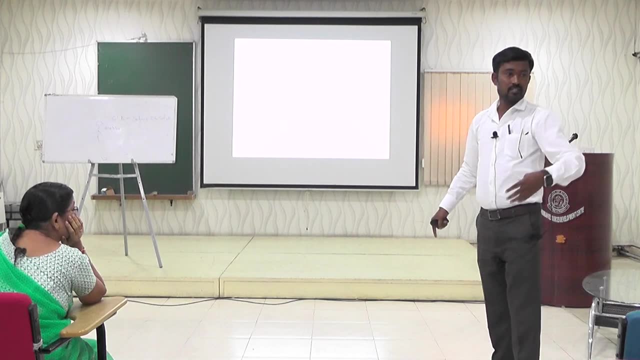 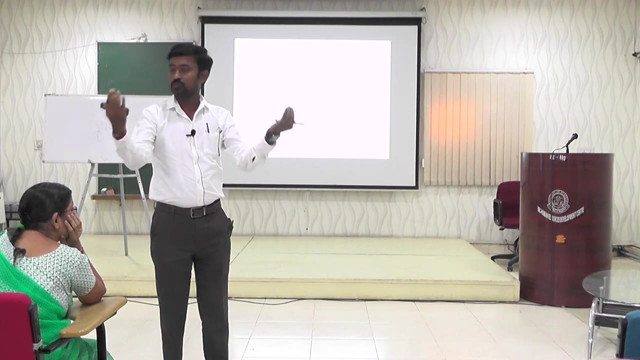 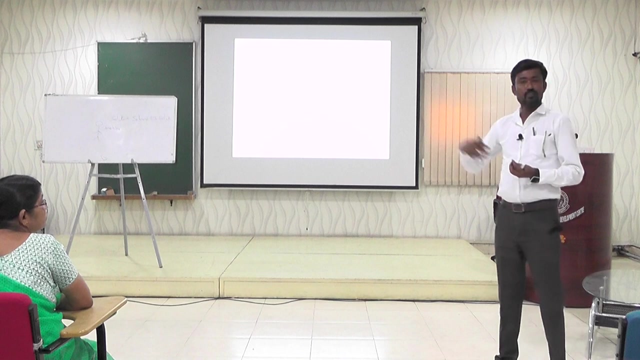 Tell What Is The, What Is The Theory Behind This, Why You Are Discussing All This- Most Of You, I Think, How You Are Sending 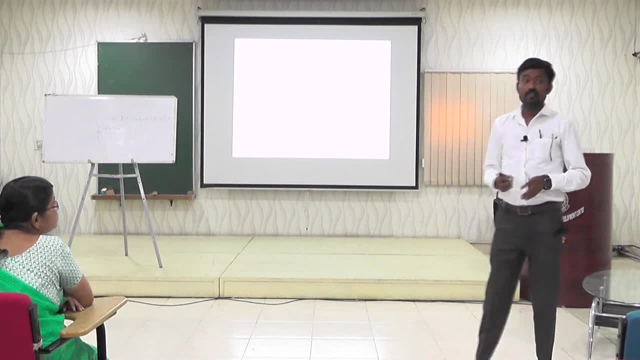 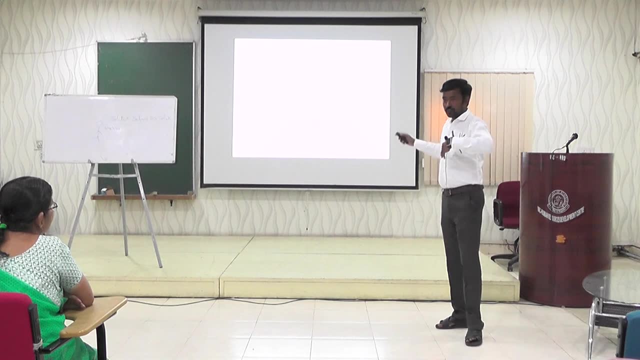 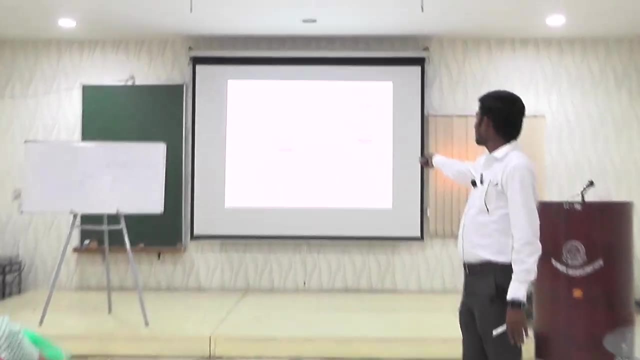 A Messages For Source Mobile To Destination Mobile: Finding A Shortest Path. Finding Shortest Path First Only, Not Only Single Path. Sometime Maybe That. 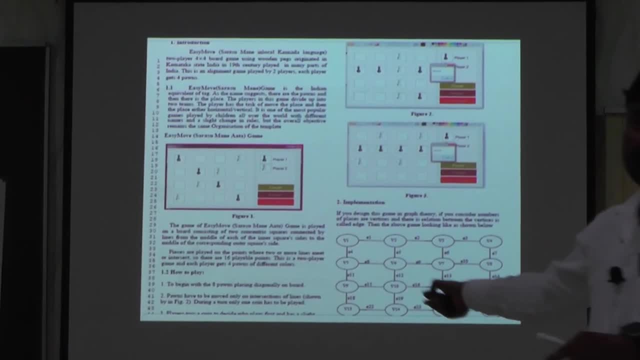 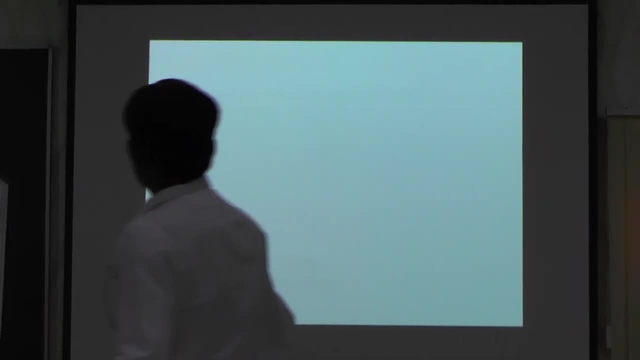 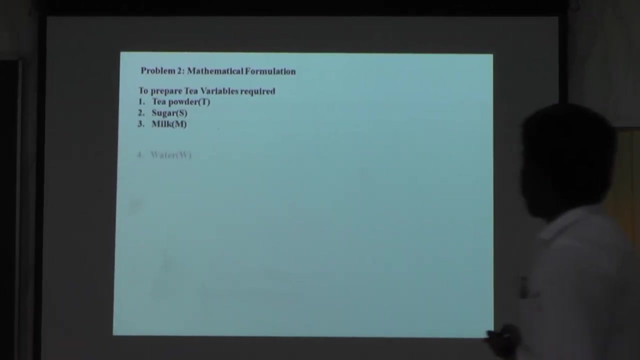 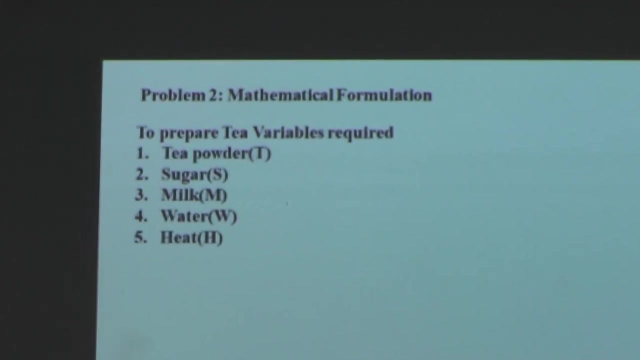 Path, Assuming That Money, Canada, It is Not A Drawb, And I Have Published This One Paper Little. Now We Know What Is Prepared, T Prepared. 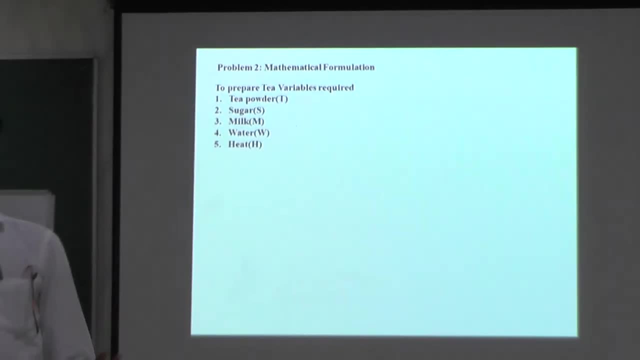 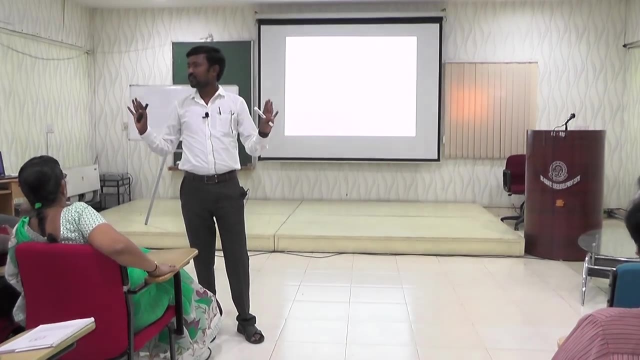 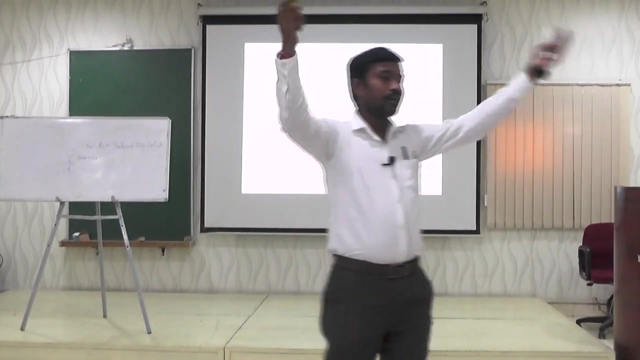 What Are The Variables Required? Our objective is to convert real world problem in a mathematical form. Is it okay? Okay, Ekta's assumption is: you need one home and so many things It is not out of. okay. 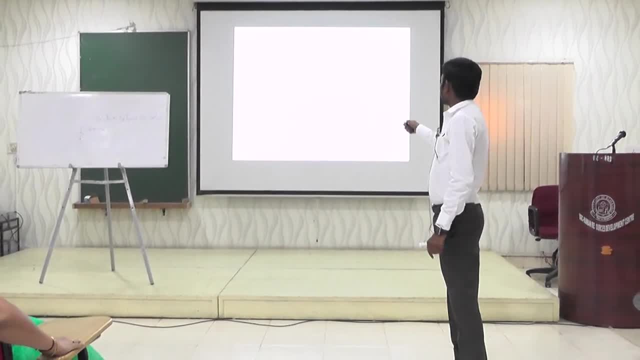 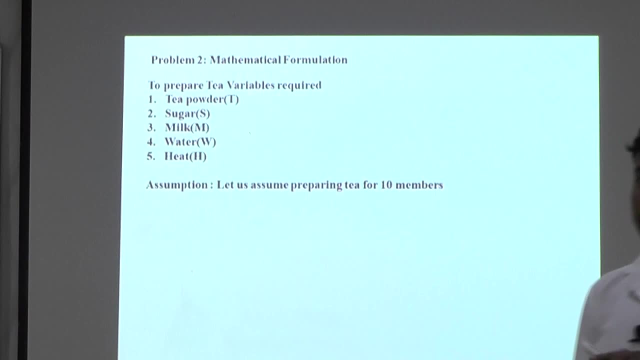 Come to the point please. I have only two more minutes. I want to complete this one. Let us assume, prepare a tea for ten members Means what you are adding ten spoon of sugar or in, I think, Andhra Pradesh ten divided by two.